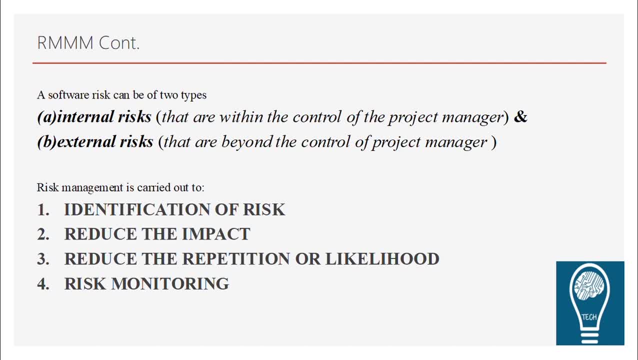 So normally what happens is internal risk as something which a project manager can plan, avoid at times, you know, reduce the impact Or, maybe you know, make sure that in case of a risk failure, we can overcome this in a very simple way. 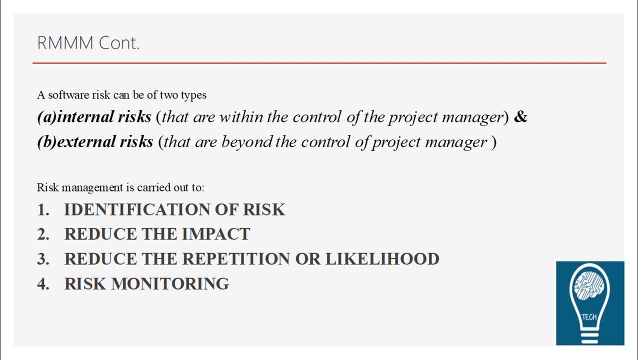 easier or sometimes, at least in a known way, whereas external risk are something which are not in the capabilities of a project manager. so risk such, as you know, government changing or maybe affect due to prices, technological upgrades and so many things. so, basically what? what are the purpose of risk management? why do we do this? 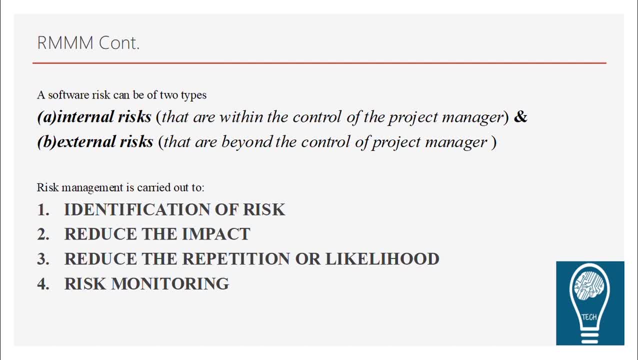 so basic idea of risk management is, to you know, first identify the risk, because until and unless we could identify the risk, we could never overcome those procedures. next step is, you know, once we know the risk, we can reduce the impact. so as soon as we know the risk, there is a planning which 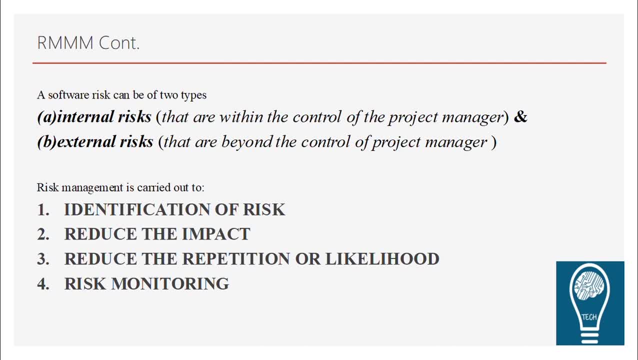 comes into picture. there are steps we take and then this is how we reduce the impact. as soon as you know, we know on the risk, we can also plan to avoid the reputation of those risks. also plan how you know likely. this is supposed to come into picture again. 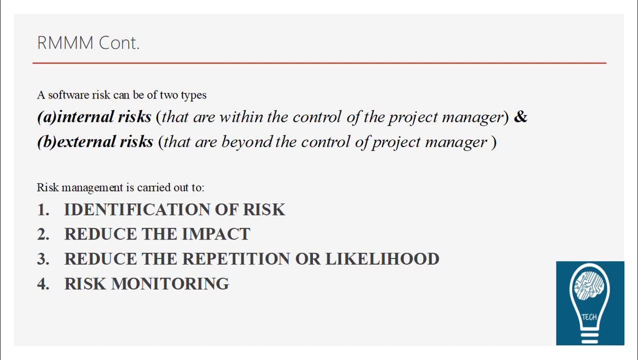 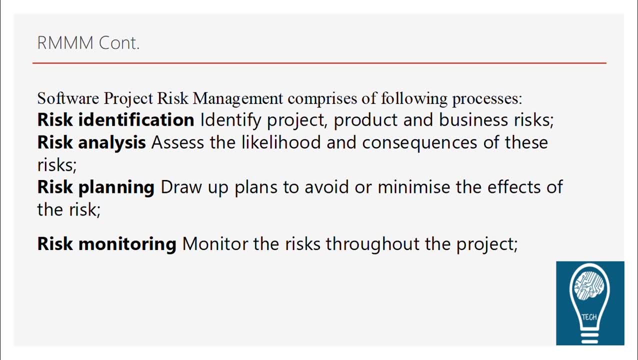 and then, as I mentioned earlier, we can always monitor the progress in order to, you know, avoid those risks. so, basically, you know this process of risk management software project. risk management involves four important things: identification of different types of risk, then risk analysis, wherein we, you know, find out the 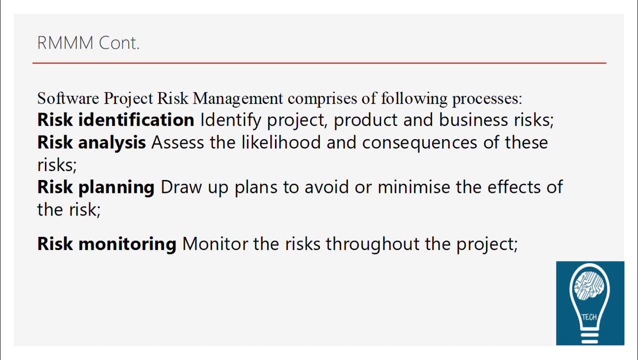 consequences or likelihood or occurrence, you know- scenarios, the planning to make sure that the effects are reduced to maximum- sorry, minimum level and also to ensure that whatever risk or you not involved, we are knowing all about them. and then, finally, that throughout the project we ensure that this are, you know, in our control. and this is how it looks. 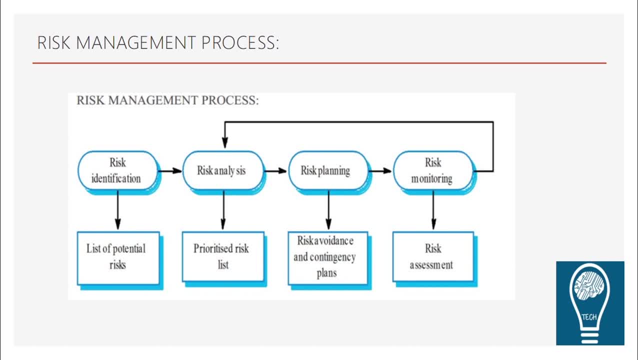 like this is a diagrammatic view of, you know, this identification, where it will list all potential risk, from technical to social to business impact and different types. then the analysis to give the priority to different risk so that the checklist can be performed and then you can avoid the occurrence of 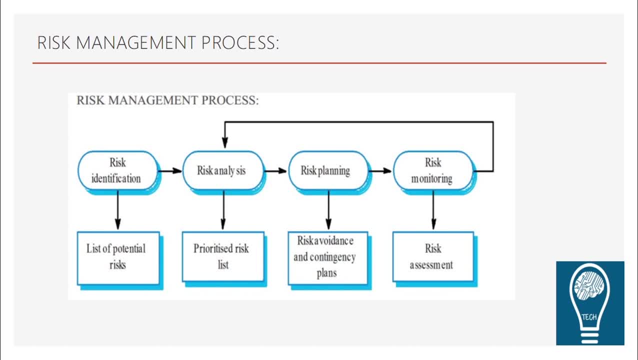 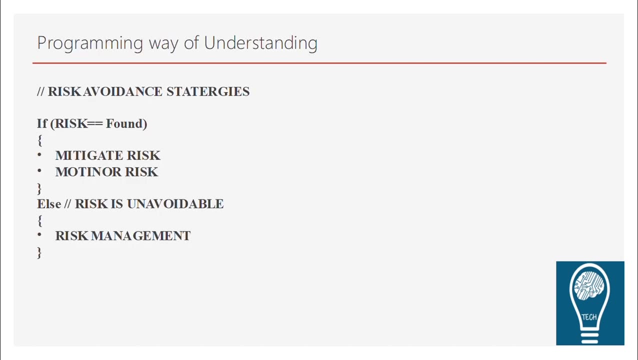 those lists. then there is, you know, planning to avoid and contingency plans, backup plans and such that, and then finally the assessment, and it's a feedback process. it's an ongoing process, so you come to know about that and you know- this is my way of explaining this in a programmatical way- that if you are 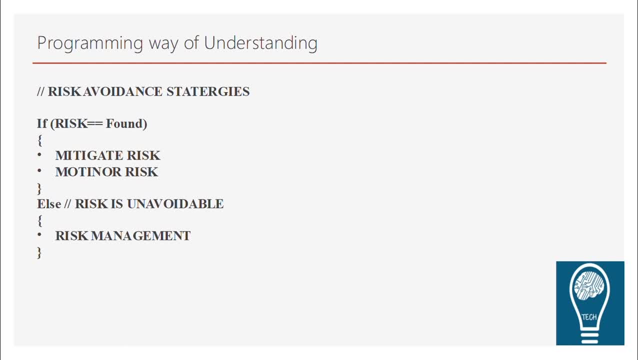 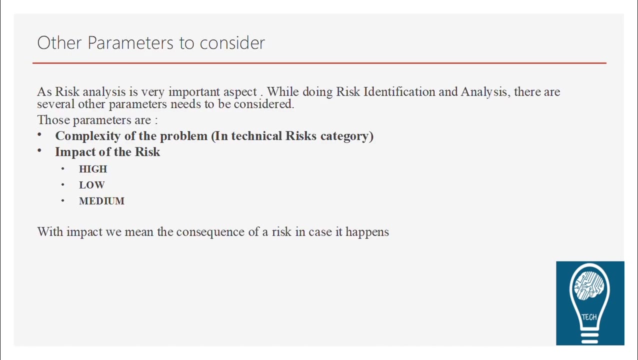 trying to avoid risk in a widened strategies. so if risk is going to found, then you do the two tasks of mitigation and monitoring. else, if it is like unavoidable, go into the management mode and reduce impact. risk management is a very complicated process. normally this task is to be performed by project. 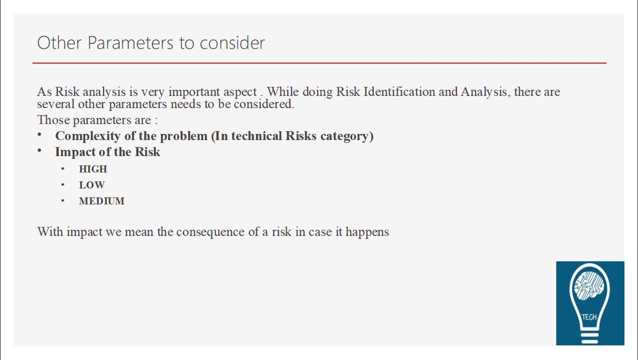 managers, software analysts and senior people, so they know what are the parameters of risk management and what are the parameters of risk management to consider. but because you might be doing it for the first time, so you need to take into account is that this analysis includes some complexity of the 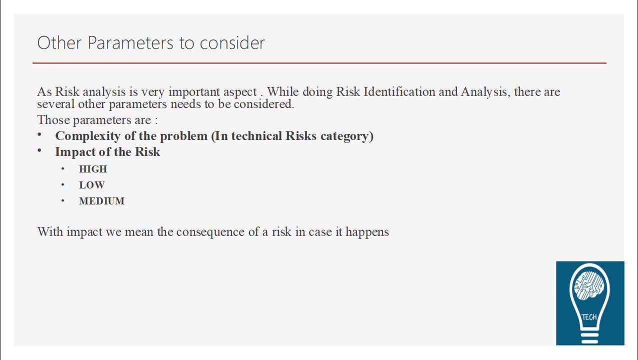 problem into account. also, we have to keep in mind different parameters and the most important part we take into account is the impact of the risk. so there is a technical risk which is a very high impact risk. we have to consider this as a very high priority. there is a risk of you know a. 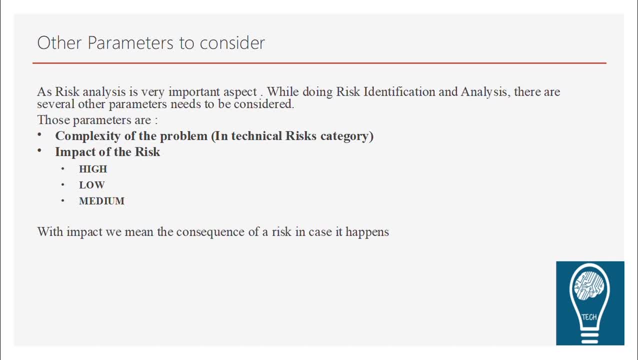 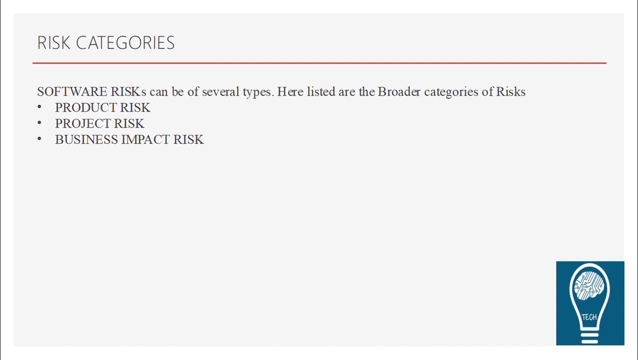 person leaving the project and it's very low, then accordingly it's tackled. so there are different risks and they are tackled and planned in a man you can say: manage using the impact of the risk mentioned with them. and what are the categories of the risk? if I were to say I would say there are three types of 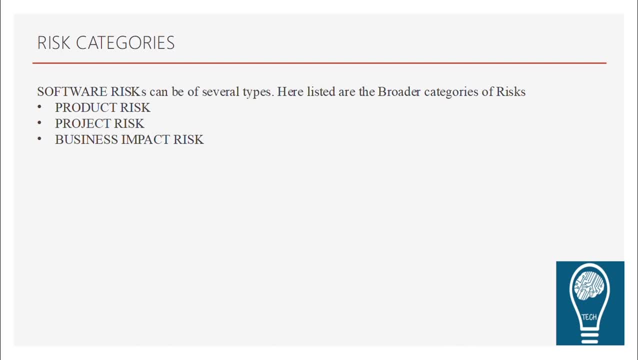 risk. one is product risk normally, which is related to the product which you are developing, and whatever the issues or the technical limitations related to the risk to the product comes in are listed under the product risk. more broader or the higher category is the project risk, where the overall project may fail. so you 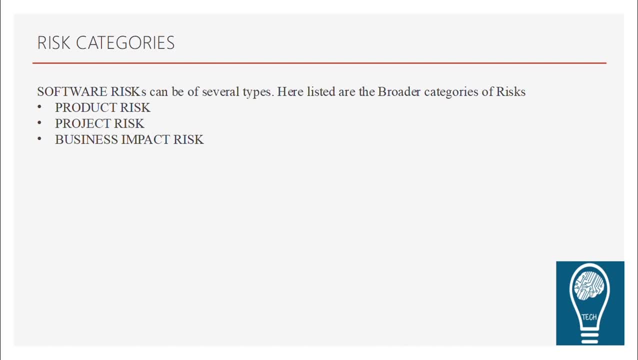 can put them into higher priority, high impact risk and the most you know important one, because when we say software projects there is a monetary terms associated with that. so business impact is the largest part of those things. so business impact risk are considered the most important ones. so these are the three basic categories of software risk. 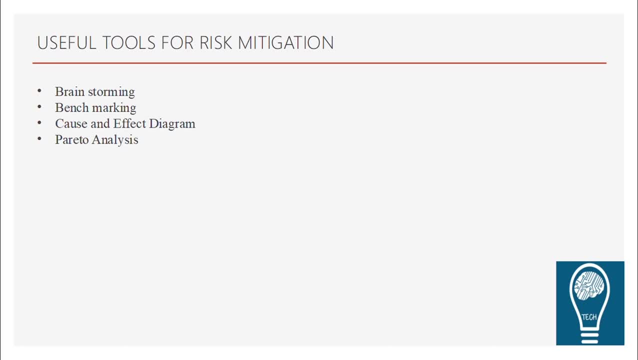 and, the most important part, how do I avoid them? so in normally software industries, they brainstorm, they plan, they execute and they even, you know, do the task in a way where it's asked for the schedule and, as you saw in our earlier videos, also of scheduling, that every task has a deadline and number of 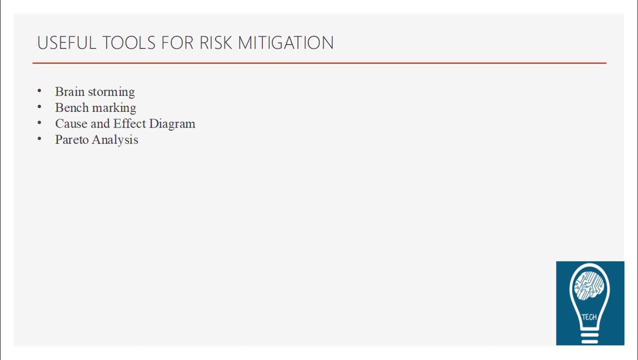 people associated and you know everything is connected. so when you brainstorm you get those ideas very clear. other techniques are also there. you can create cause-and-effect diagrams just to come up with more understanding of those lists. certain tools are available in the market. so whatever I'm suggesting is, at a basic student college level, a process which 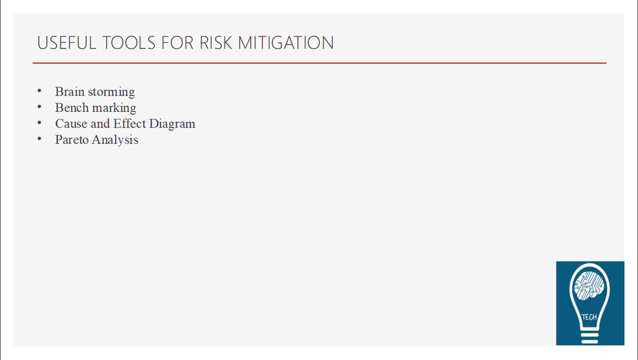 you can do to mitigate as you go corporate. there are multiple tools, multiple techniques available which you can do. as I mentioned, you can even perform Pareto analysis. so this is a basic idea of what RMMM is all about, and this can be applied to a lot of different types of software. so this is a basic idea of what RMMM is all about and this can be. 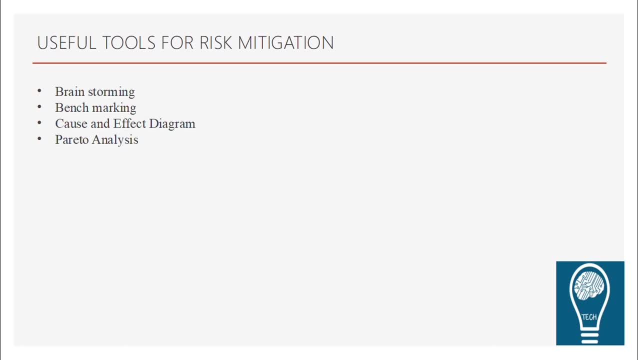 applied to different projects. you need to understand your projects very well in order to do this, so I think this would be quite helpful for you to understand. what is this mitigation monitoring and management plan. I hope you would have understood this and now you can go back to your projects and perform them for. 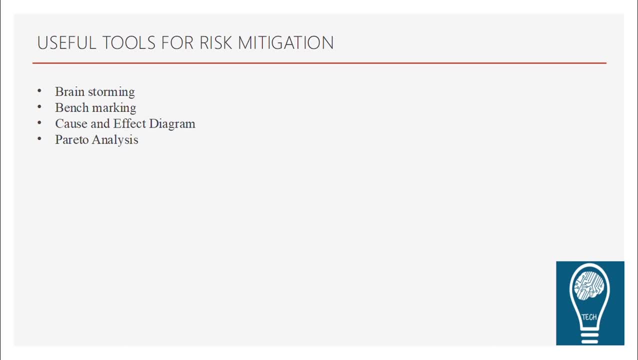 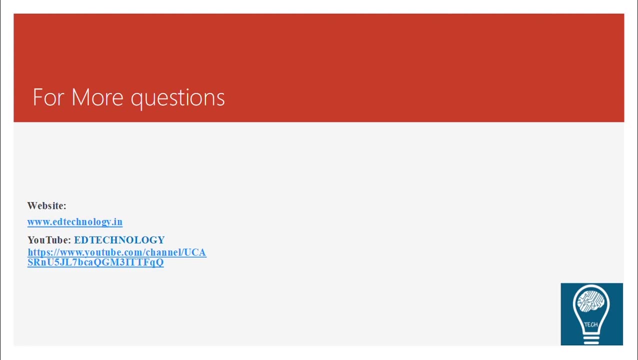 any queries. you can always comment in our comment section and thank you for your time. please subscribe our channel, ED Technology, to support this initiative of educating more people. we are planning to educate everybody on computer science for free of cost, so that is the whole idea. thank you so much. do subscribe our. 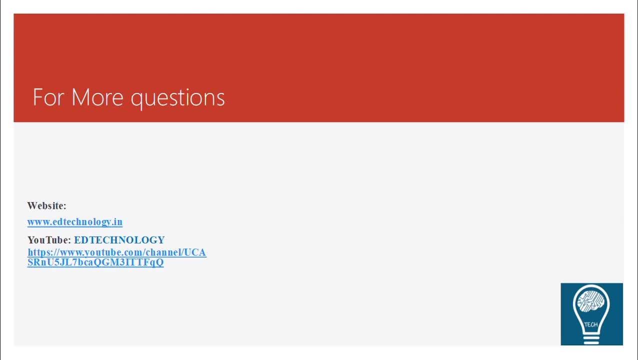 channel. it's Navjot saying: hasta la vista.